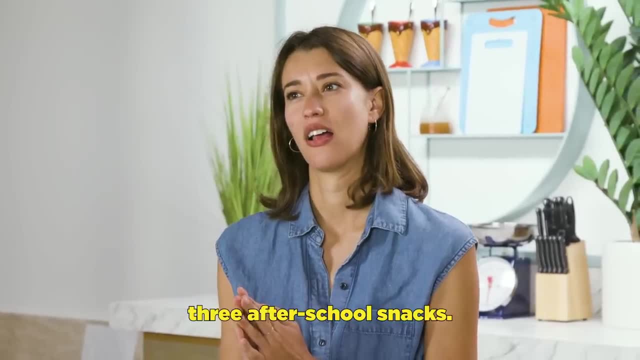 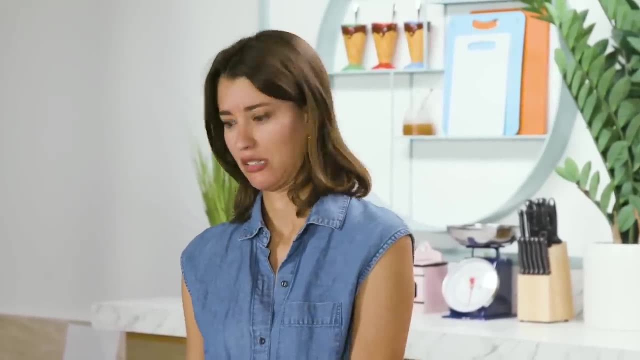 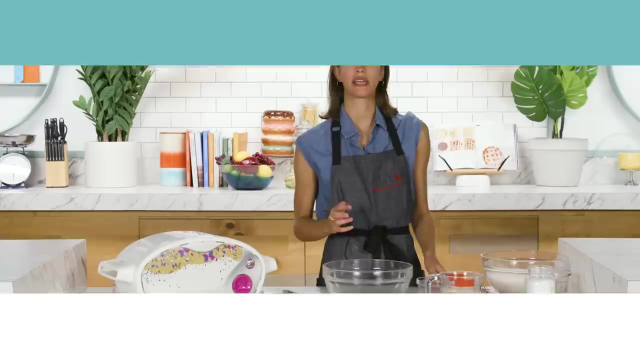 Oh no, Okay, It's gonna be fine. It's gonna be fine. I think I have a plan. We'll see if it works. For the first course, I'm going to make a personal pizza. To make it really delicious, I'm gonna start off making my own dough. 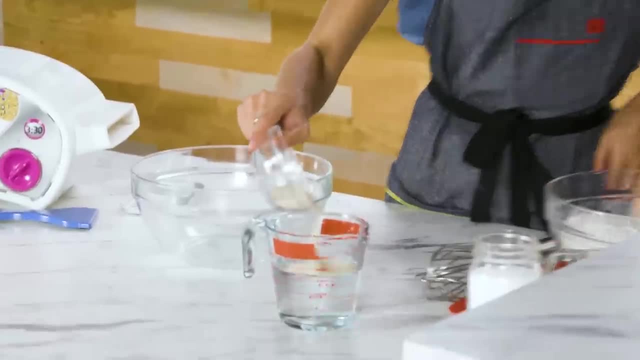 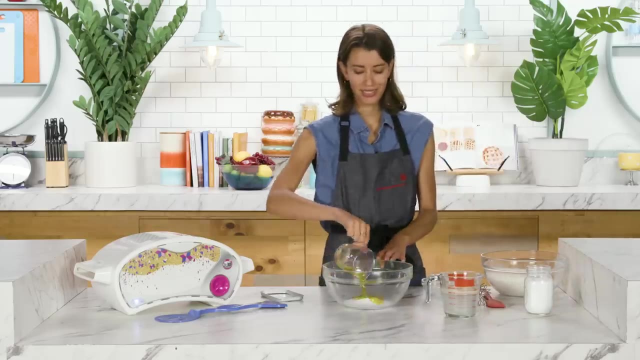 So I've got my warm water. I'm gonna sprinkle some yeast over it and let it bloom. In the meantime, I'm gonna whisk my butter, My sugar, salt and olive oil. This is gonna be a really simple, quick pizza dough. 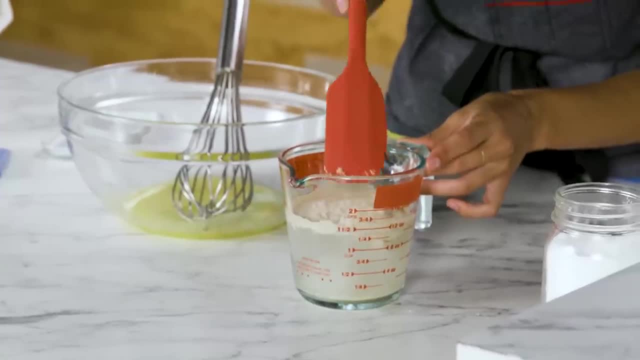 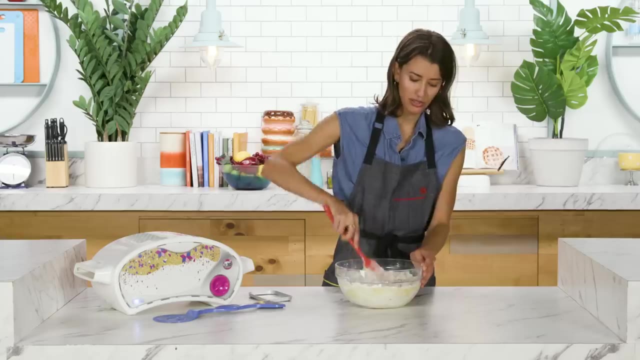 You can tell when the yeast is blooming, because it'll start to bubble. a little. Yeast looks foamy and good. Gonna add that to the oil And adding the flour. I just had the thought that pizza usually cooks at really, really high temperatures. 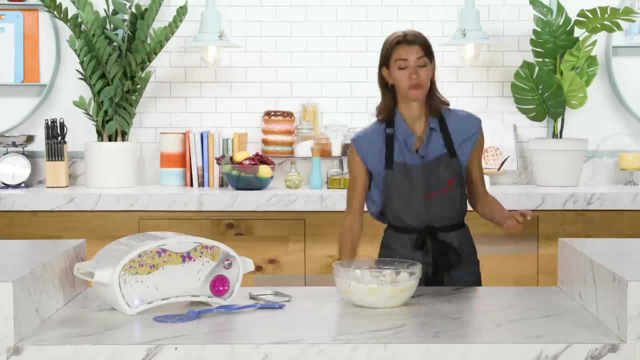 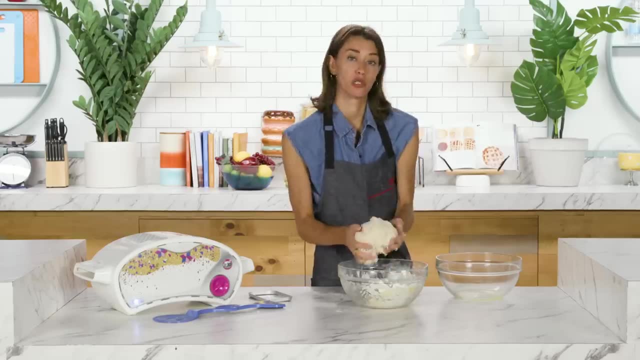 The internet told me this only gets to 350, so pizza dough might be a bad idea. Maybe, if I roll the dough out super thin, I'm gonna let this rise in this oiled bowl. While my pizza dough rises, I'm gonna get started on my next course. 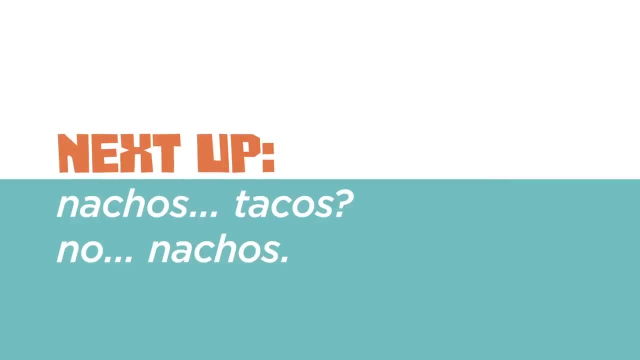 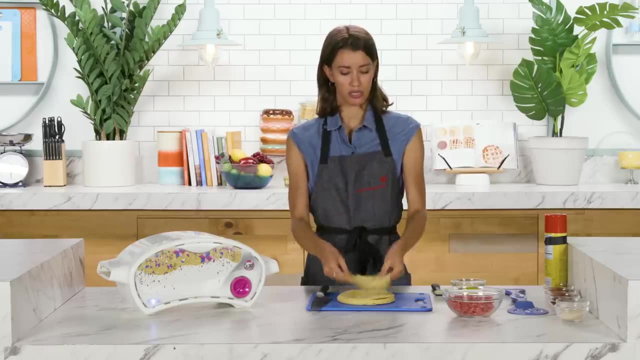 because it's gonna take a long time. For my next course I'm going to do nachos. I had this idea that I could make my own tortilla chips by just cutting the tortillas, brushing them with oil and hopefully they'll crisp up in the Easy-Bake Oven. 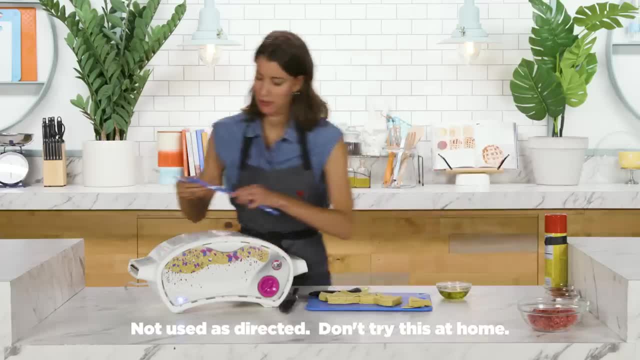 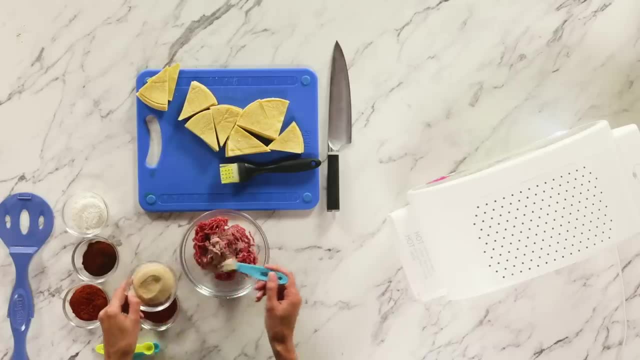 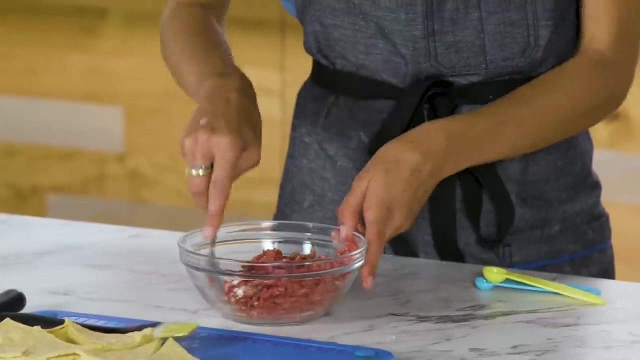 Let's see how this goes. I'm gonna add some spices to my ground beef: Some salt, garlic powder, onion powder, chili powder, paprika, cayenne, And I guess I'll just mix it. Ground beef needs to cook to 160 degrees so it should be able to work in here. 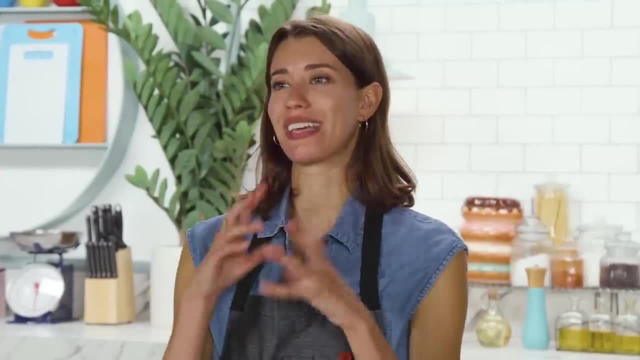 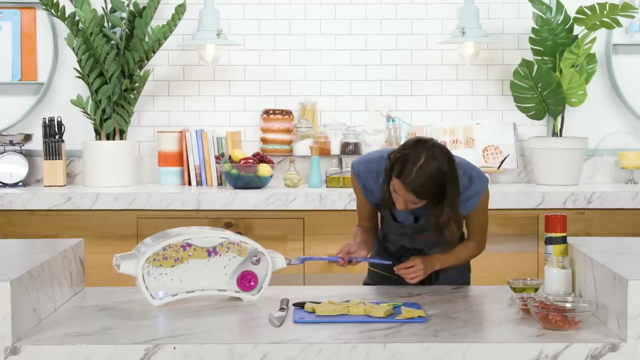 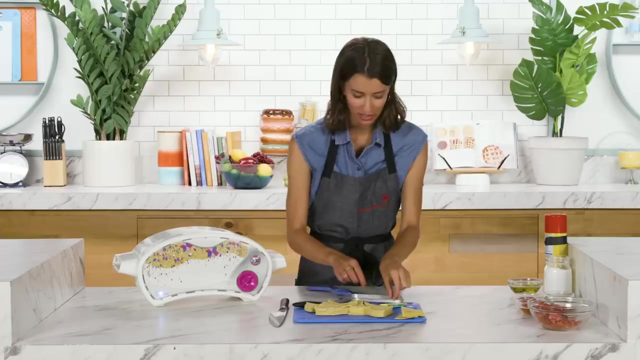 I just don't know how long it'll take. and again, I don't think it's gonna get that browning. I have a feeling it might be kind of gray. I'm gonna check on these chips. Ah Okay, it's not quite there, but it's actually kind of working. 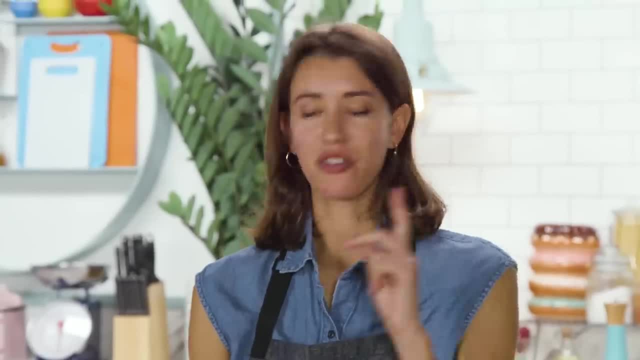 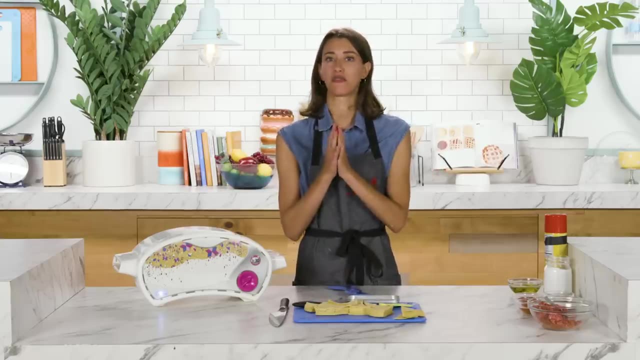 Like there's some crispiness here, Okay, but here's the thing: It's gonna take me like three hours just to make chips. Is there any way that I can have some help? I have a lifeline for you. 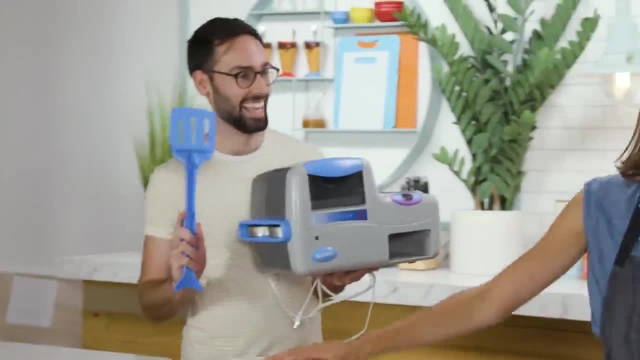 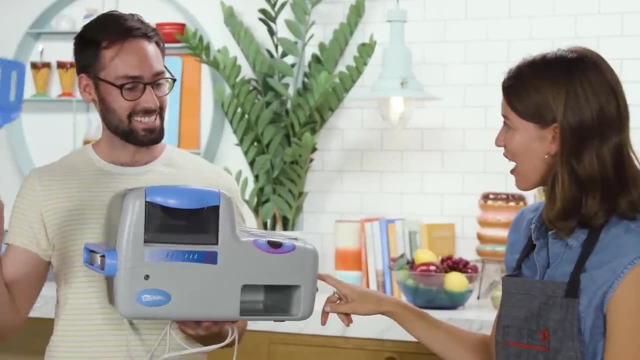 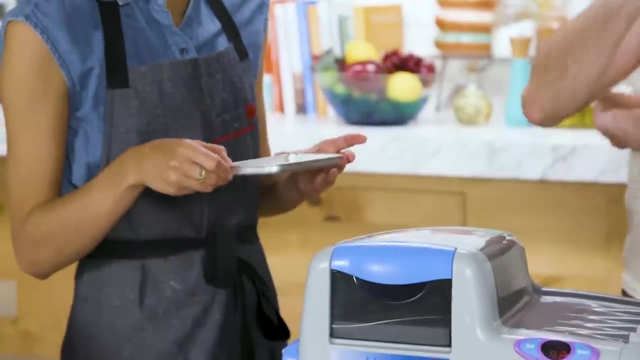 Meet your sous chef. Oh hi, My sous chef turns out to be my best friend And I got one too. Okay, so, the first step, we have to preheat it. Okay So? Oh, I know this is crazy, but we have to do it like two chips at a time. 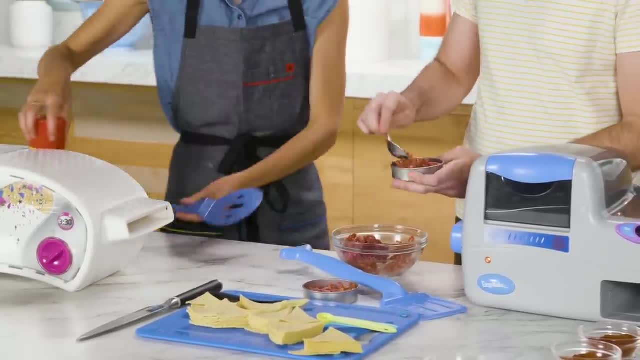 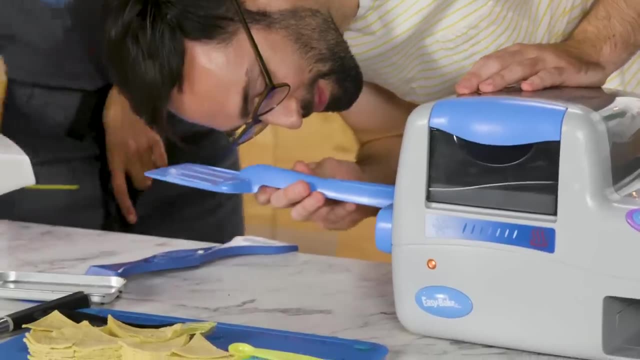 Okay, I think while I work on chips, I'll have you work on ground beef. Oh okay, I really want to use this. Got it, Okay, Got it. I heard that. I mean, how crispy do you need chips to be really? 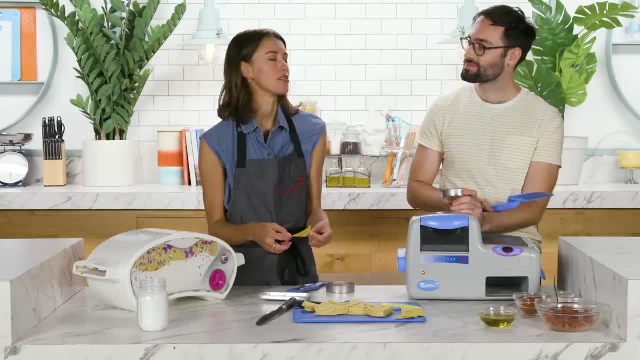 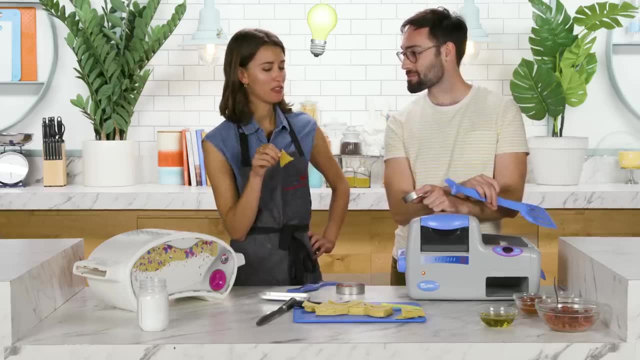 You know what? I think we can pivot to mini tacos. That's cool. I think it's time to check. Okay, Oh Ooh. It's like: Oh, wait, And I can do this. Oh my God. 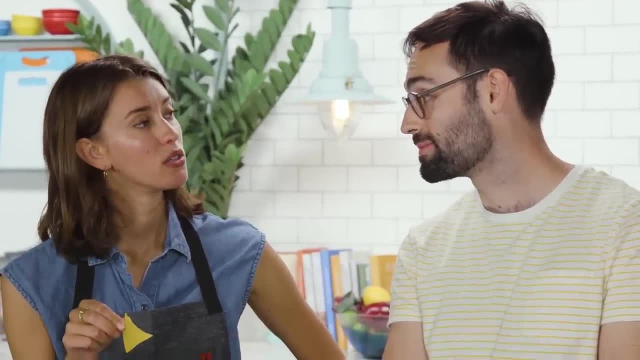 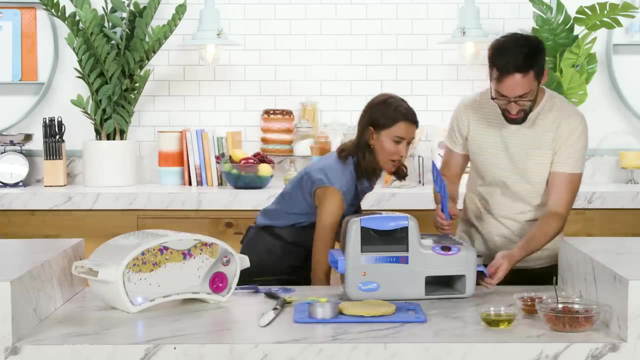 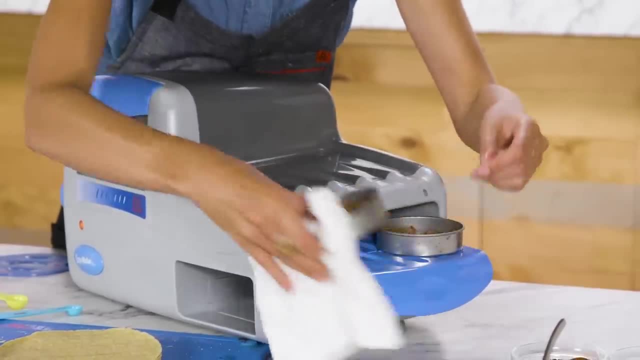 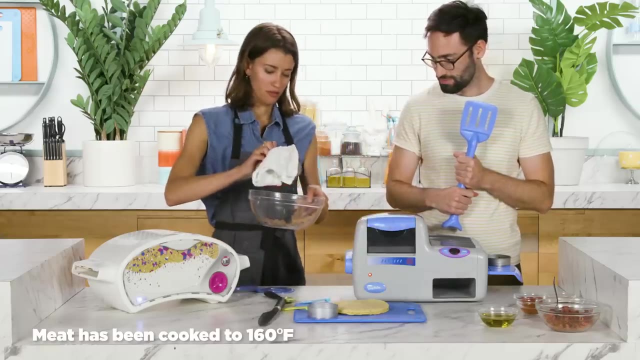 Okay, Wow, Okay, This is. This is kind of cooked. I know, Holy, I'm shocked. Okay, We have a long way to go, Uh-huh, But I think if you keep doing the beef, Yeah, we'll be good. 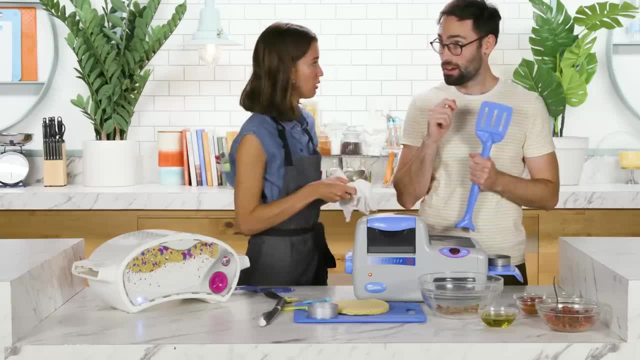 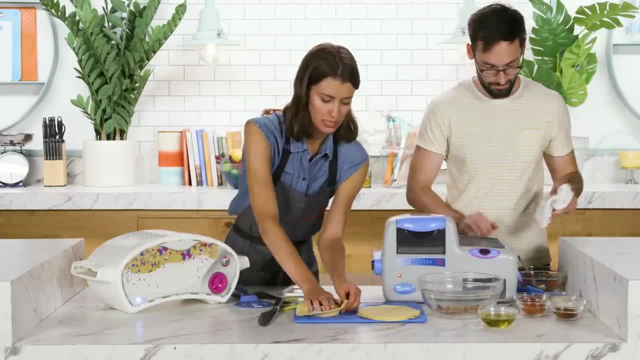 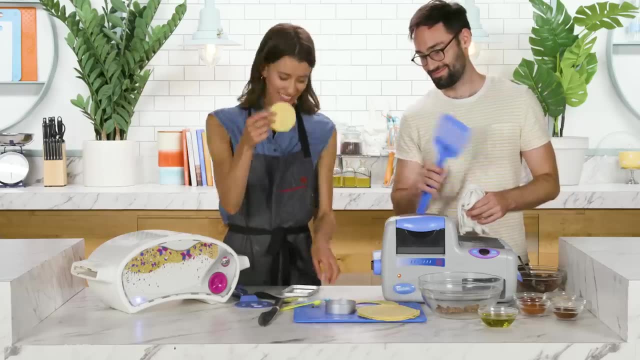 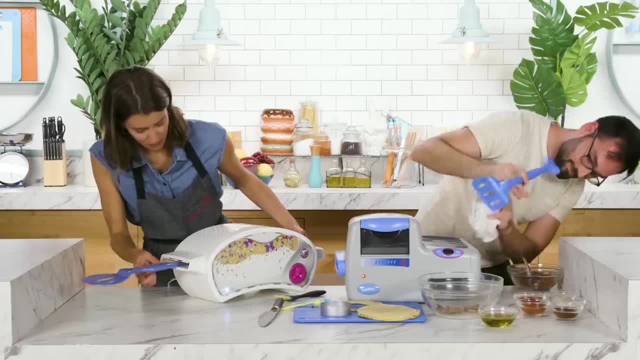 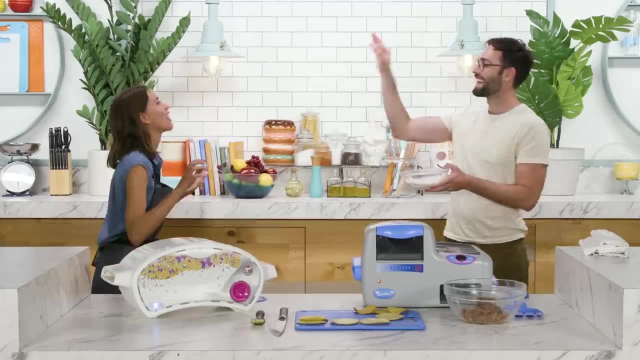 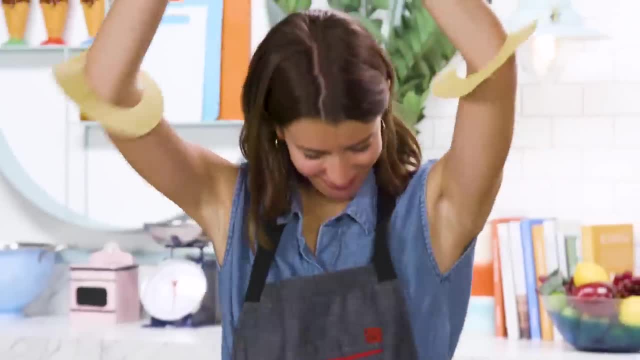 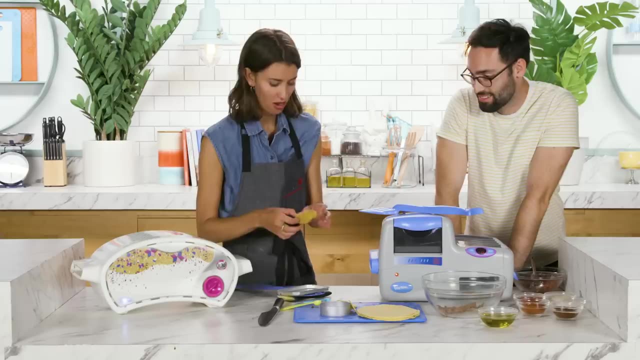 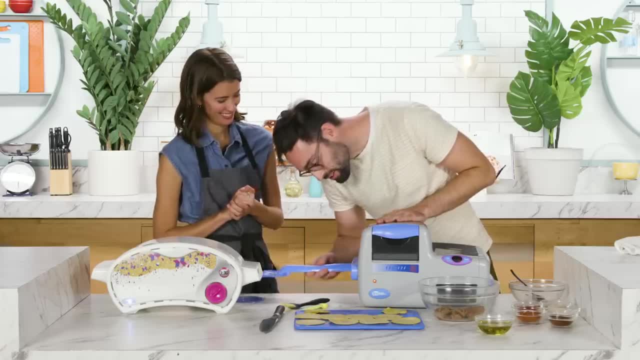 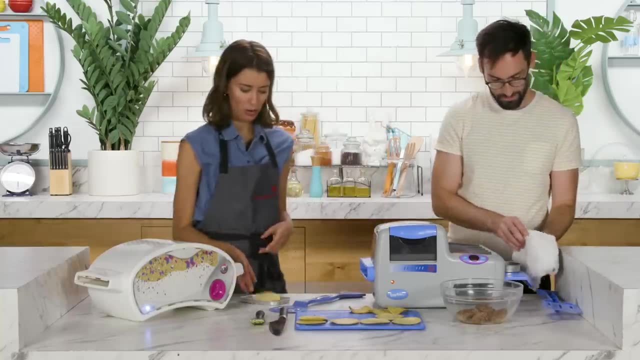 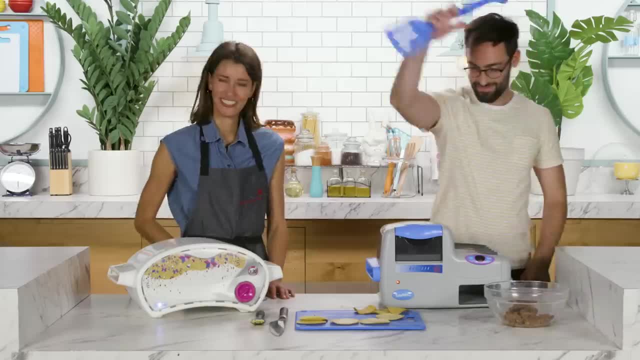 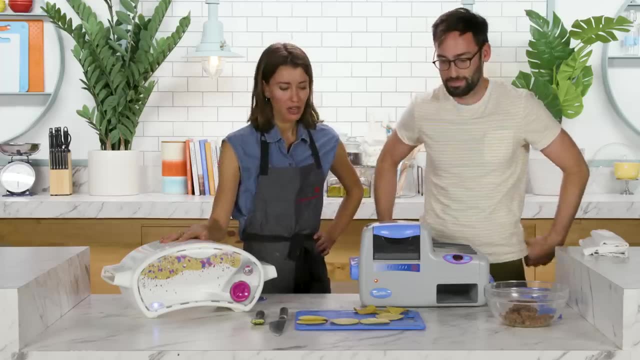 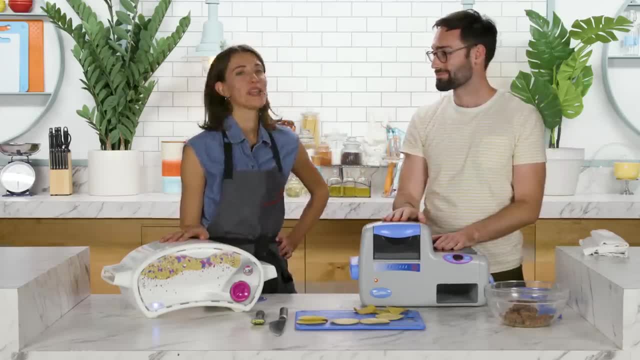 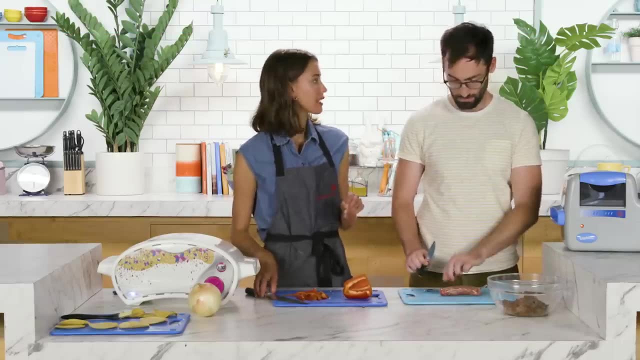 We're actually almost at 10.. It should only take 25 more minutes For the personal pizza. One sausage: Okay. if you can remove the casing and crumble it up, gonna do it the same way that the ground beef, Okay. 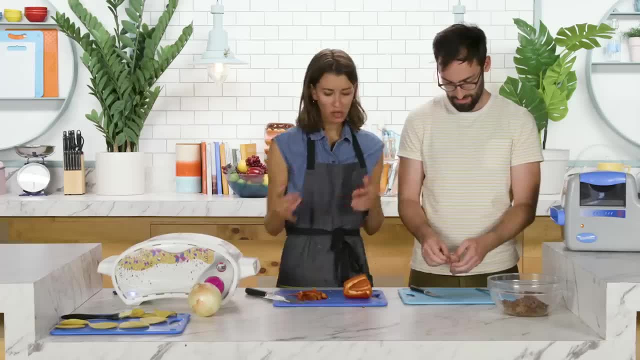 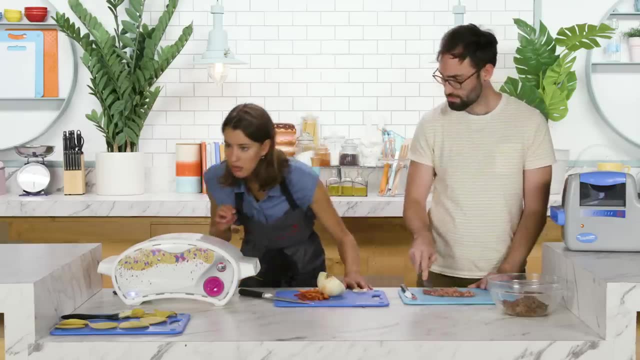 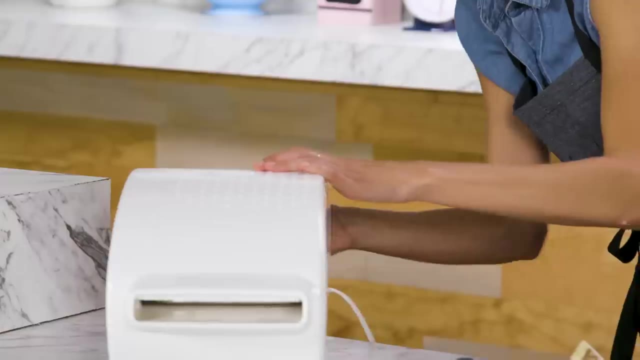 I was thinking of sausage, pepper, onion pizza. Feels a little ambitious now, but I think the pepper and onion can just be will kind of roast. Wait, Oh, this is smoking. Uh-oh, Okay, One very crispy chip. 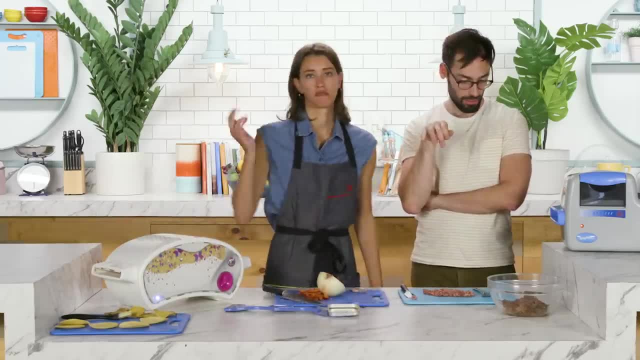 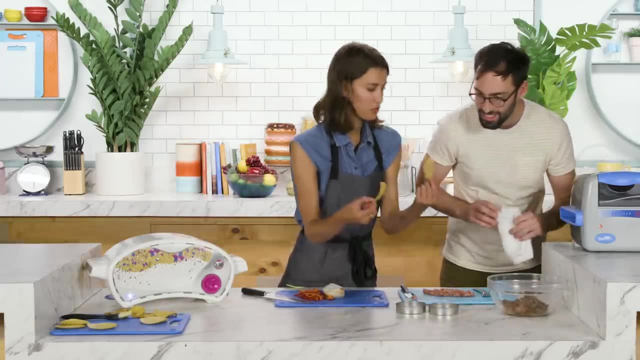 You know it's fine. It's fine, It'll be on the bottom of the pile. Some people, that would be their favorite chip. Yeah, What do you think Yours are beautiful? Ooh, Sorry, Two chips Love it. 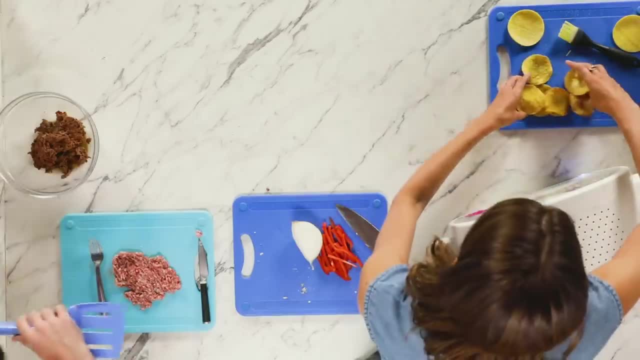 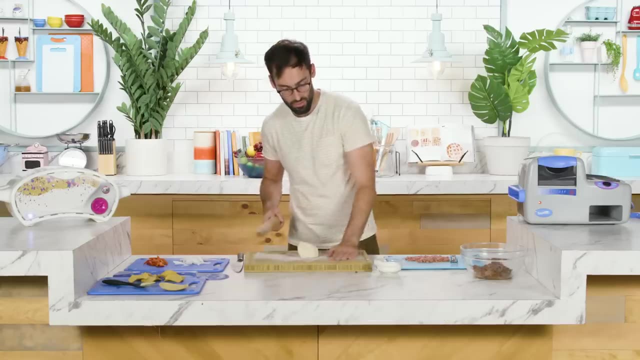 All right, All right, I'm gonna do nine chips. That feels sufficient. Ooh, wow, This dough is Wow. It's feisty. I think she's doing well. I think we're coming to the part I'm nervous about. 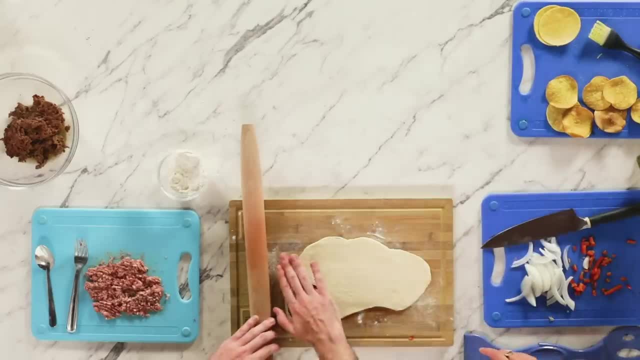 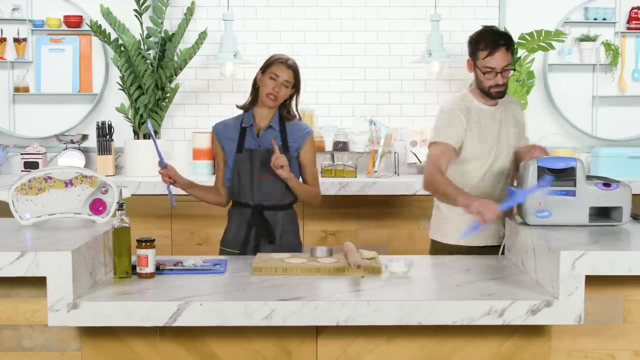 Okay, if you can get that cookie cutter and stamp out two Circles, Circles. Okay, can you check the sausage? I bet it's done. Mm-hmm, Mm-hmm. I'm gonna check the peppers and we'll see where we're at. 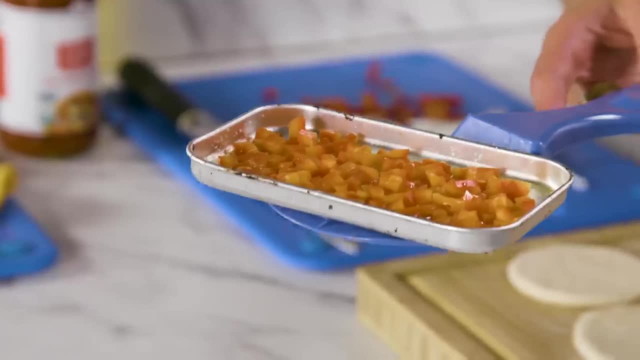 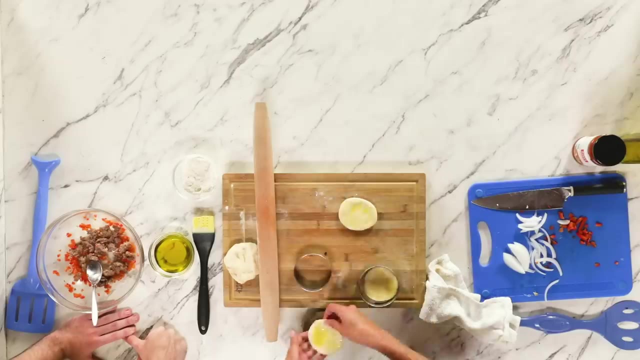 All right, Oh Ooh, look at the peppers. Do you think the sausage is ready? Woah, Yeah, Amazing, Amazing. Okay, Do you want me to do it? Do you want to do it? The honors. 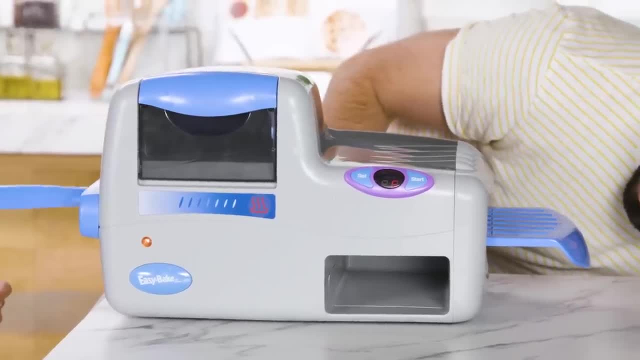 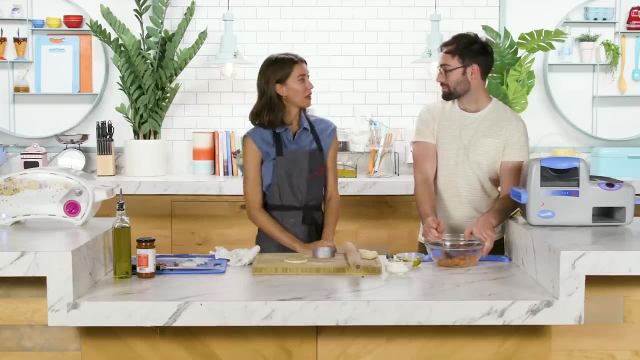 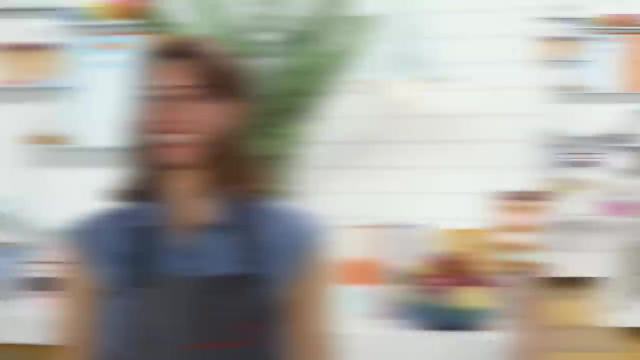 It's like a real pizza Here. I'll check this. My confidence level about the pizza is a seven. Cool, Oh, you seem. No, I'm happy for you. Thanks, Can you check the pizza? Gladly. I just took these onions out. 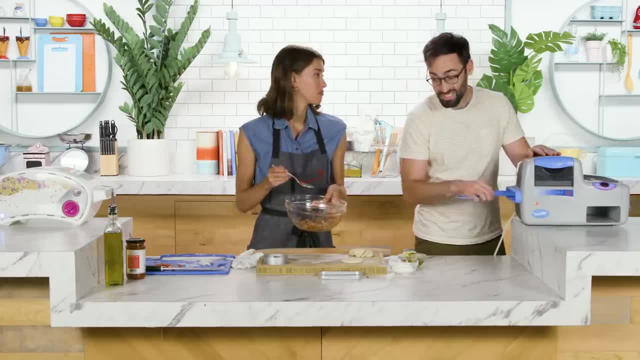 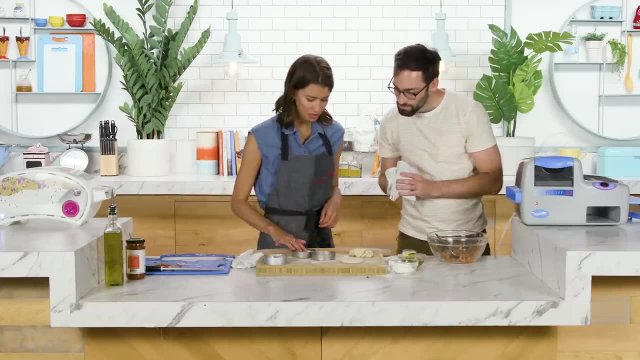 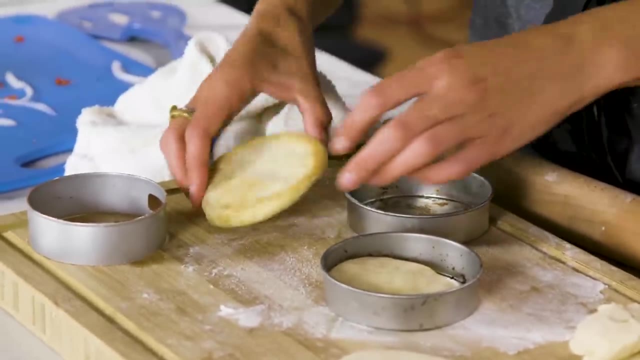 We have it actually looks. it looks really good. It smells good too. It smells like very doughy, Right. Yeah, Oh, okay, Okay, these look, these look amazing. I mean this is, yeah, Wow, cool. 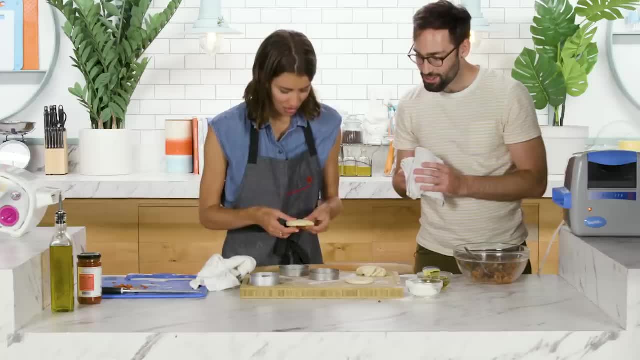 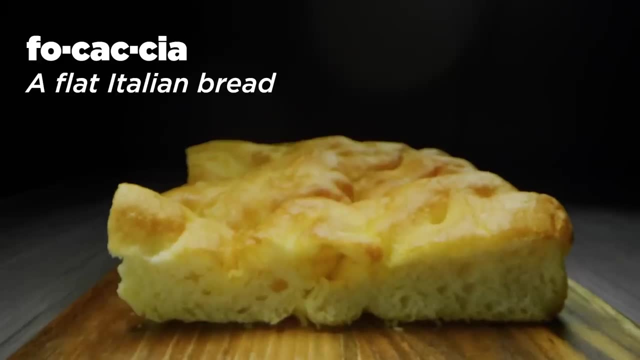 Oh my God, the bottom has some brown. So what They're? I mean, this smells. it smells amazing. It's kind of more like focaccia than pizza, but That's great, It's fine. I think I have it from here. 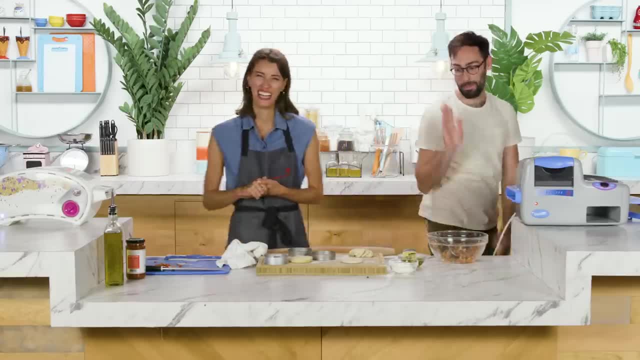 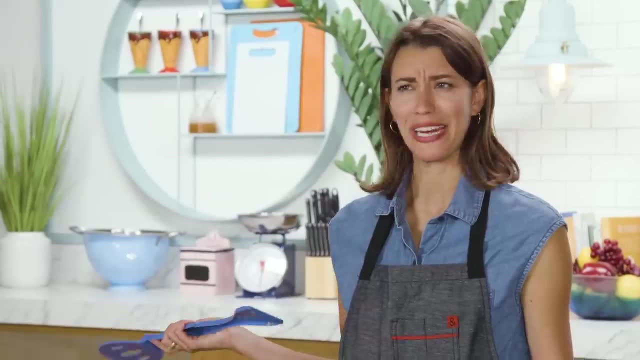 All right, Thank you so much. I can't wait to see Bye-bye. Bye. Ryan was the biggest help I could have ever asked for. It's time to start plating. This is pre-made sauce. Got some mozzarella and some of my toppings. 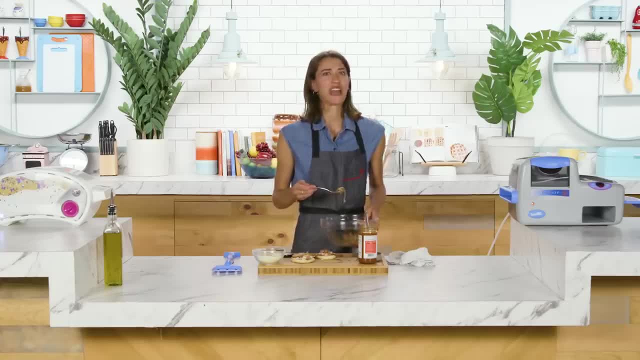 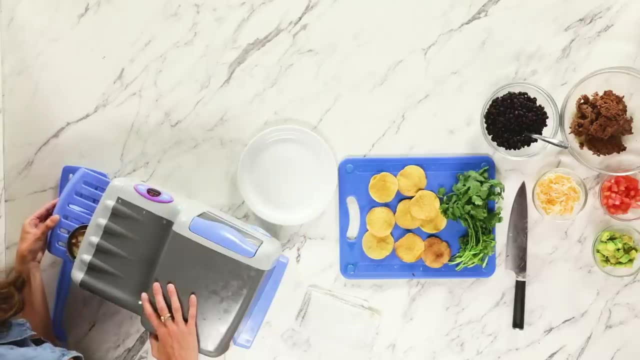 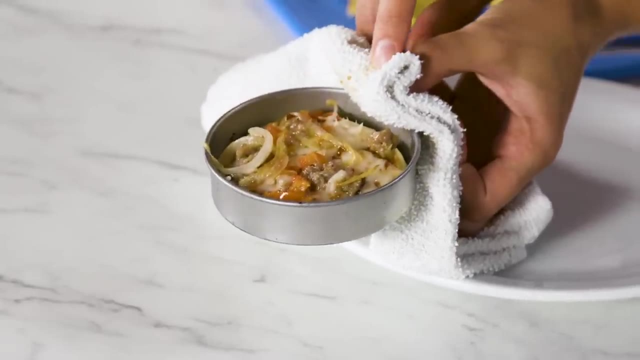 I'm so excited for this person to guess what I used, Like they're gonna have no idea. This is actually really fun. Ss, Ss. I made a mini pizza with real pizza dough in an Easy Bake oven. Making food with a kid's toy is so out of my element. 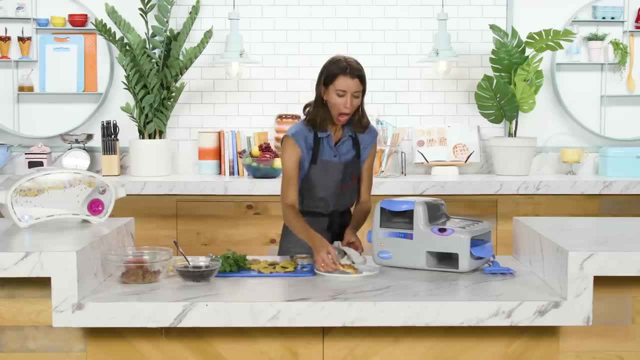 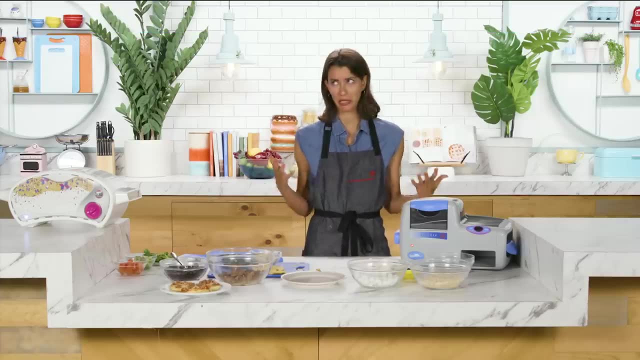 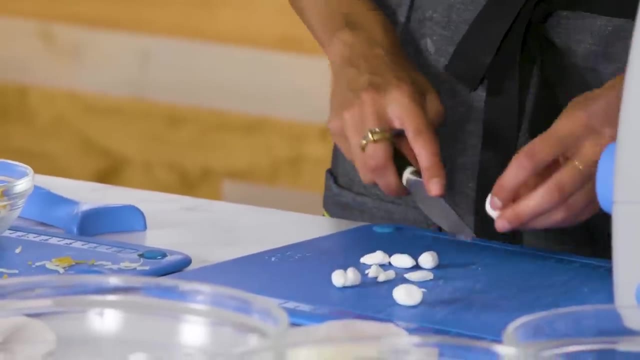 but I feel elated. There was a cheese pull, Did you see it? One of my favorite after school snacks was cookies every single day, So this definitely needs a sweet element. so I'm gonna make a crispy rice snack. I'm just gonna cut some marshmallows. 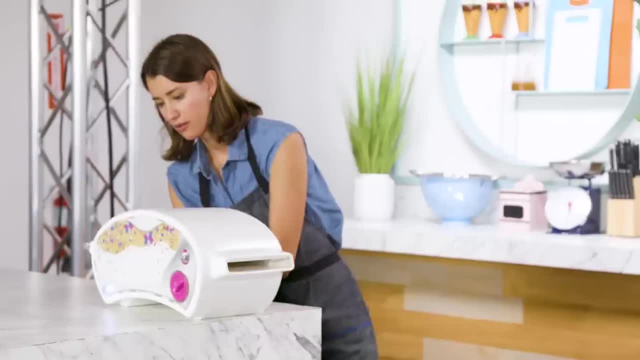 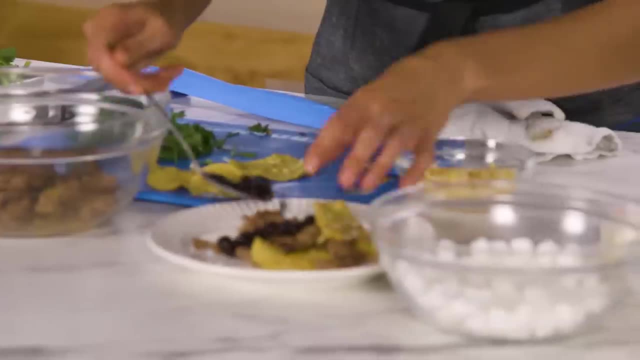 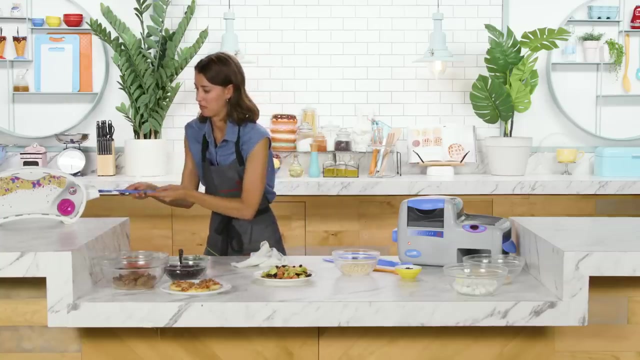 put some butter, got my marshmallows on and pop them in. I'm gonna layer the nachos with obviously chips, cheese. my ground beef Got some black beans, tomatoes and some avocado. Oh boy, Uh-oh. 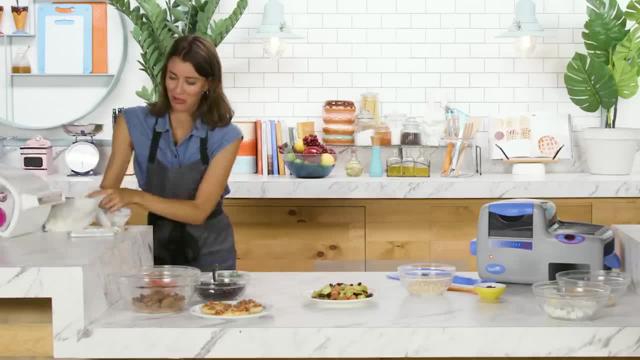 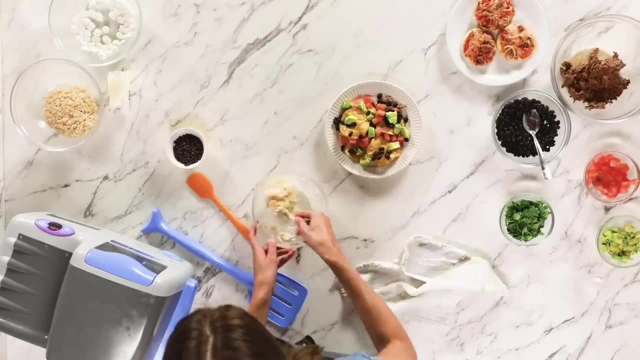 Seems to be a bit of a marshmallow explosion. Woo Shoot, okay, okay, okay, fine, fine, fine. Pressure is on This. I feel better about this. This looks good. Gonna add chocolate chips. I'm gonna go find a cookie cutter. 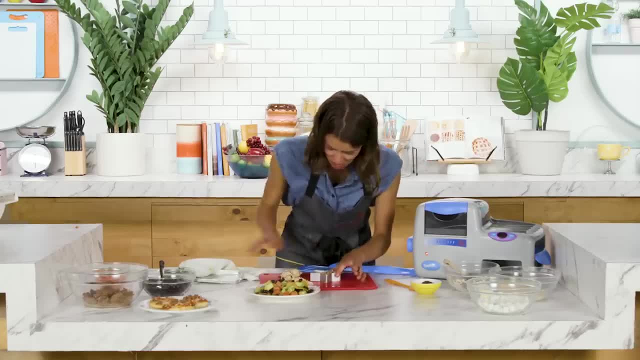 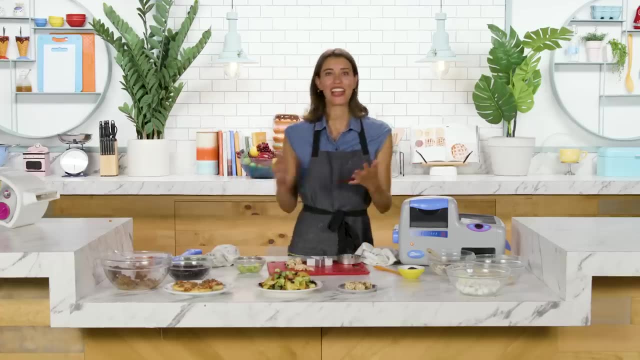 and put this into a cute shape. Oh my god, this is so cute. Okay, I've been told that the taste tester's here and they're ready to try, and I can't wait to see if they can guess what I've used. 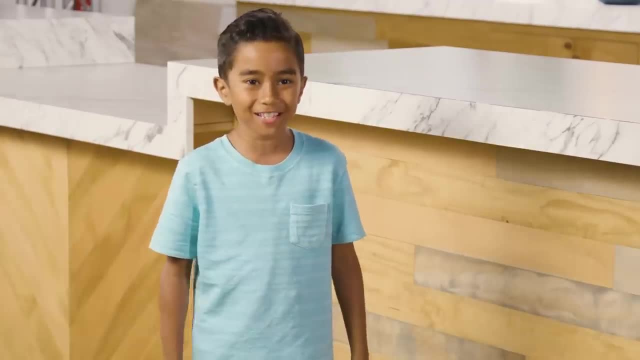 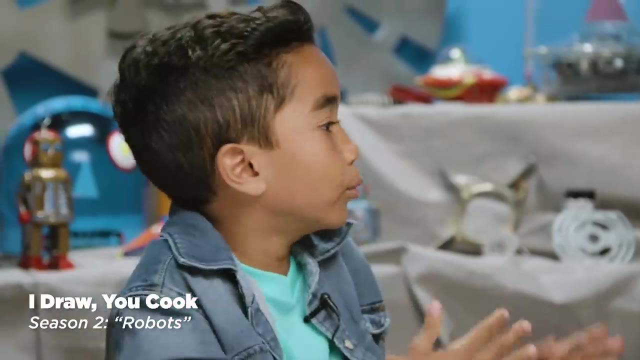 My name is Jonas and I'm nine years old. The first time Alexis cooked for me was on. I Draw You Cook robot episodes. We heard you really like robots. Beep boop, bop, bop, boop beep. 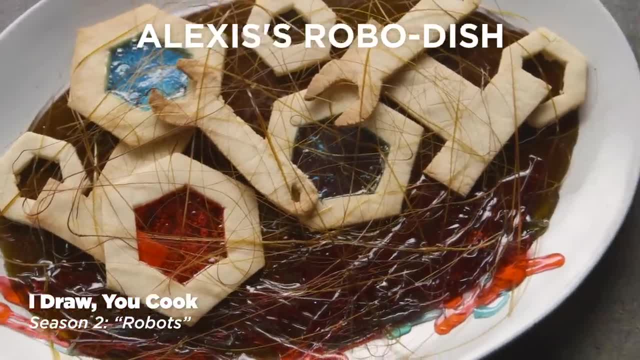 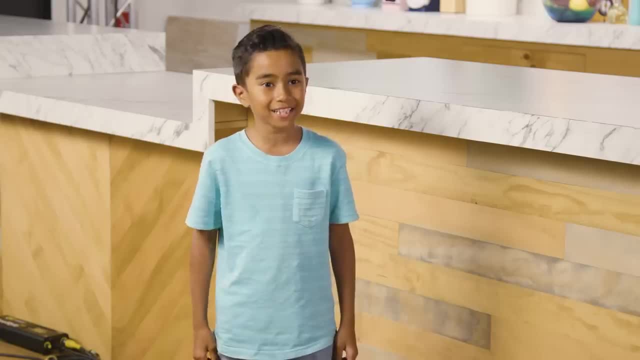 Let's eat. I actually love it. I think it looks so weird and cool. The cookie dish That's mine. That was amazing. Today Alexis made three snacks for me and I have to guess what she used to make it. 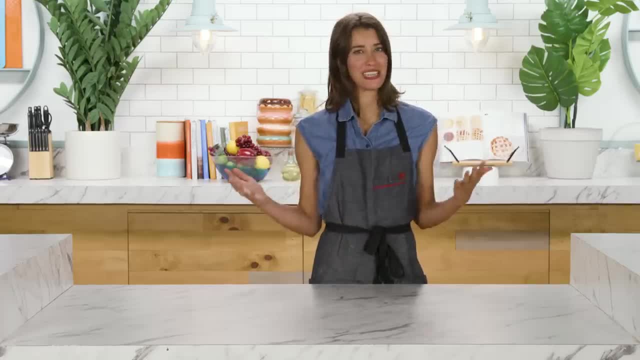 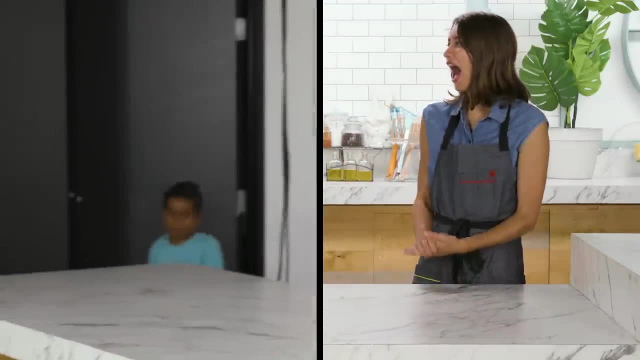 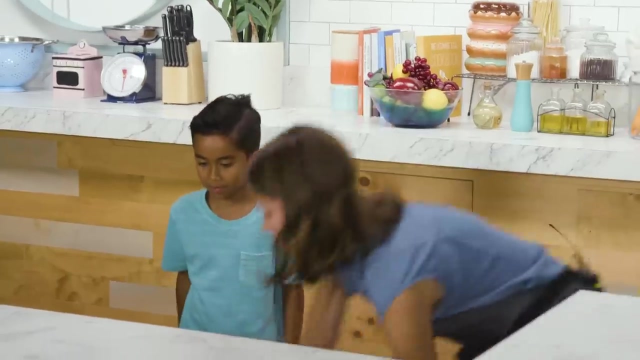 I'm so proud of everything I made and I can't wait to see what this taste tester thinks. Let's bring him out. Bring him out. Oh Hey, look, Hi High five. Let me get you something, Wow. 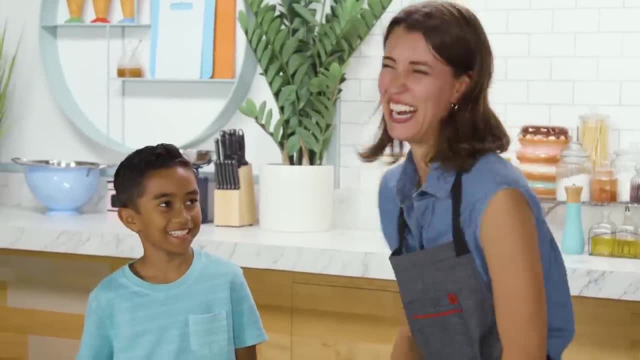 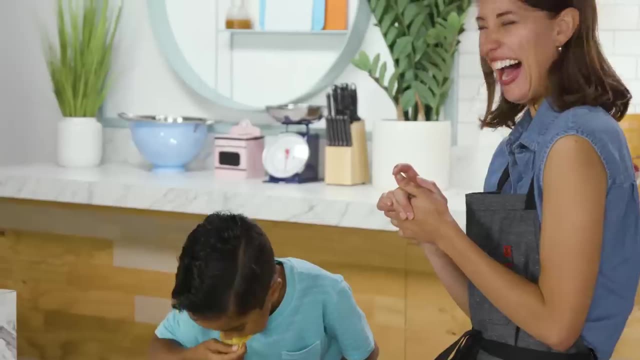 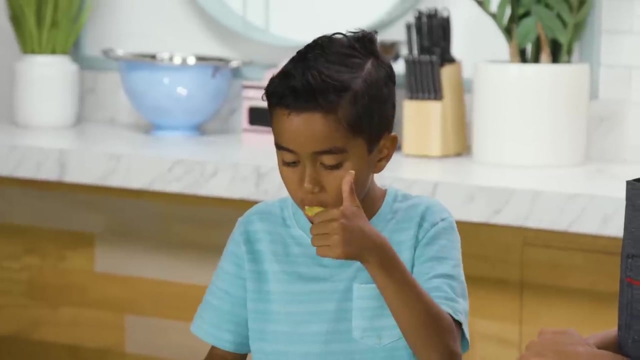 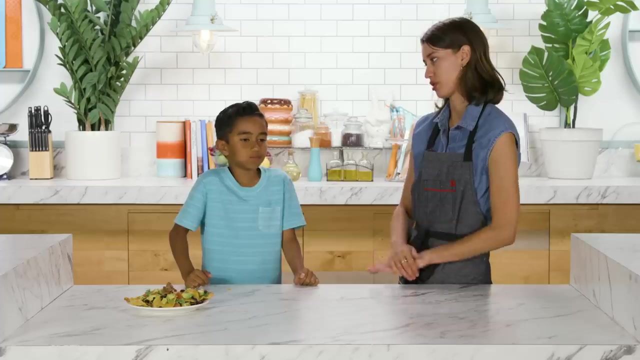 It's so good to see you again. You, too, How's it going? Good For your first after school snack. you have nachos. It's good. Tastes like nachos. Ooh great. On a scale of one to 10, what would you give these nachos? 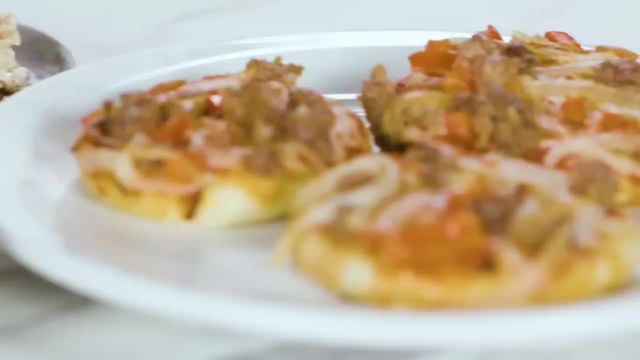 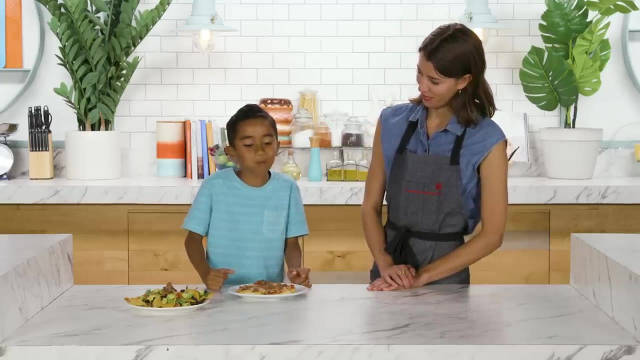 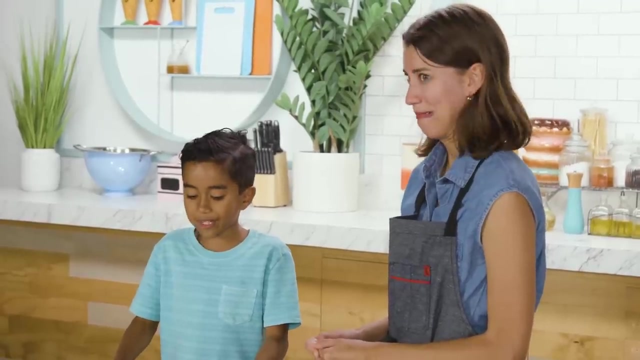 An eight. Great, I'll take it. You've got mini pizzas with sausage, pepper and onion. It's good. Does it taste like pizza? Yeah, Yeah, Maybe the crust would be a little harder. I think that's a fair assessment. 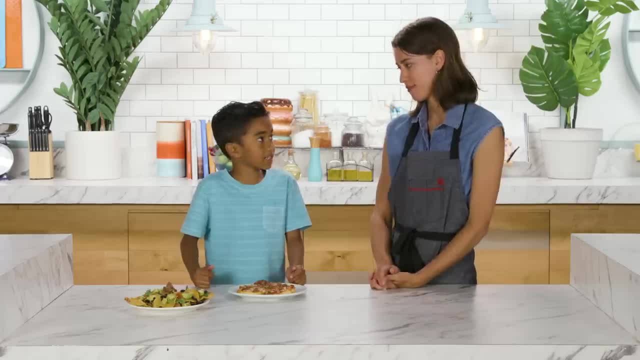 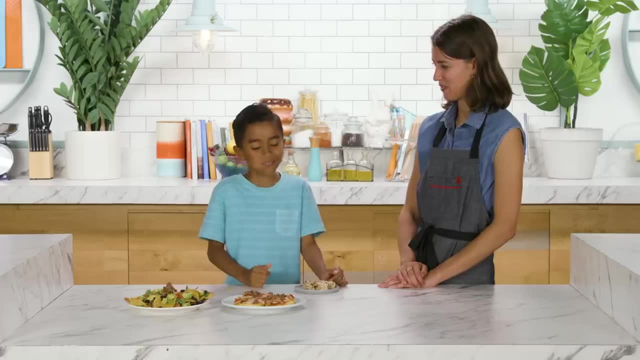 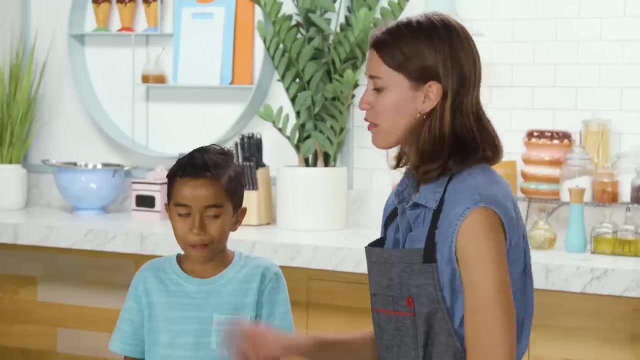 On a scale of one to 10,. what would you give this pizza? A six Fair. Are you ready for your last after school snack? Ooh, It's good, Hey. A 10. A 10?? OK, so we've got an eight, a six and a 10..